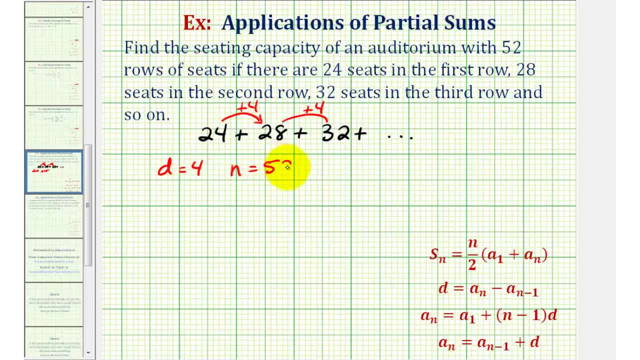 series would be fifty-two. We also know a sub one. the first term is equal to twenty-four. And now to find the partial sum of this arithmetic series, we can use this formula here: a sub n is equal to n divided by two times the quantity. a sub one. 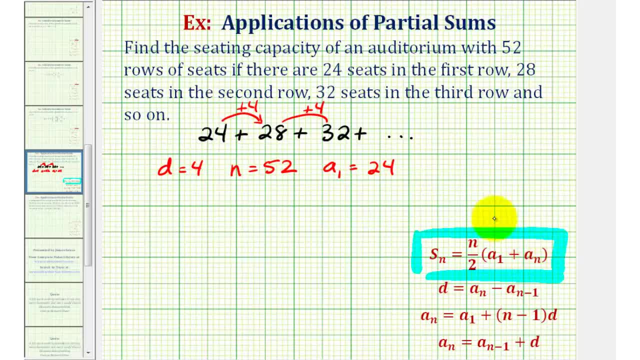 plus a sub n. So notice, before we find this partial sum, we also have to find a sub n, and since n is equal to fifty-two, we need to find a sub fifty-two plus a sub fifty-two plus a sub fifty-two. 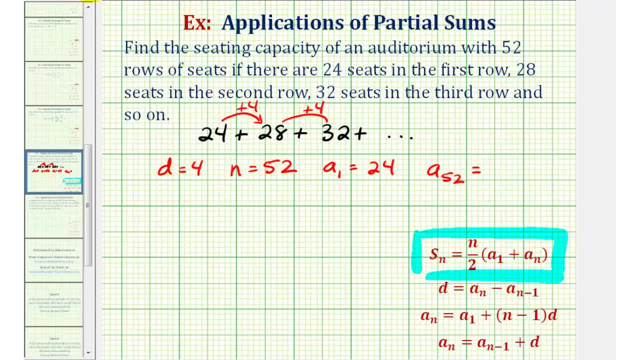 To do this we'll have to use this formula here, where for an arithmetic sequence a sub n is equal to a sub one plus the quantity n minus one times d. So let's go ahead and find a sub fifty-two, and then we can find this partial sum. 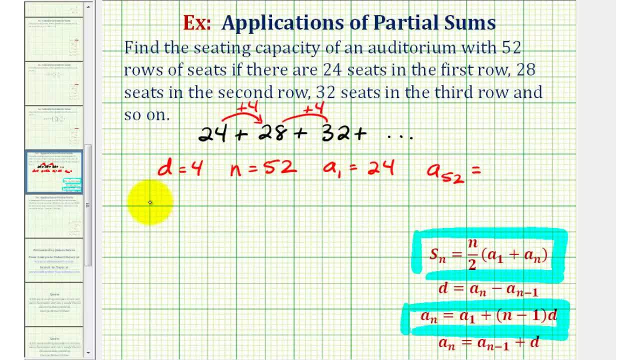 So a sub fifty-two is going to be equal to a sub one which is twenty-four plus n minus one where n is equal to fifty-two. so we have fifty-one times our common difference d, which we know is four. 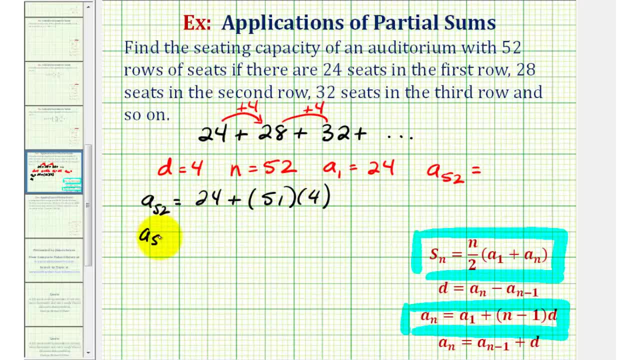 So a sub fifty-two is equal to twenty-four plus two hundred four, So the fifty-second term is two hundred twenty-eight. And now, using this information here now we have all the information we need in order to find the number of auditorium seats or the sum of this arithmetic series. 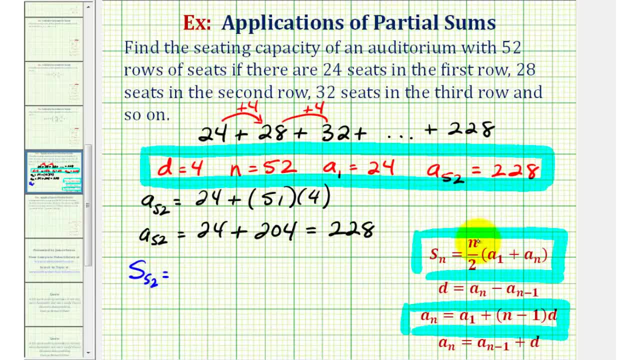 A sub fifty-two is going to be equal to fifty-two divided by two times the quantity: a sub one plus a sub n, or in this case, twenty-four plus two hundred twenty-eight. Fifty-two divided by two is twenty-six. 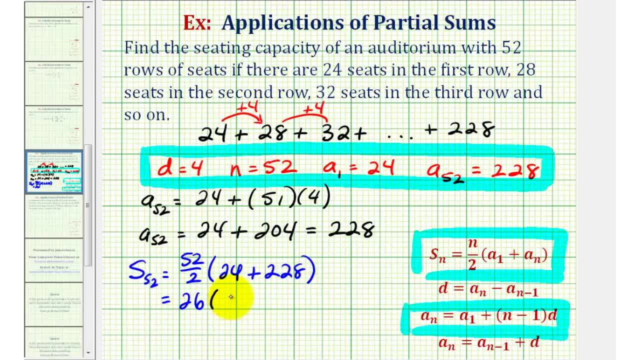 Twenty-four plus two hundred twenty-eight is equal to two hundred fifty-two, So the number of seats in the auditorium or a sub fifty-two is equal to twenty-six times two hundred fifty-two is equal to six thousand five hundred fifty-two. 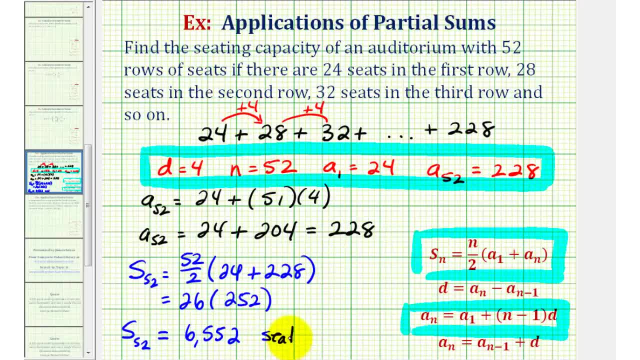 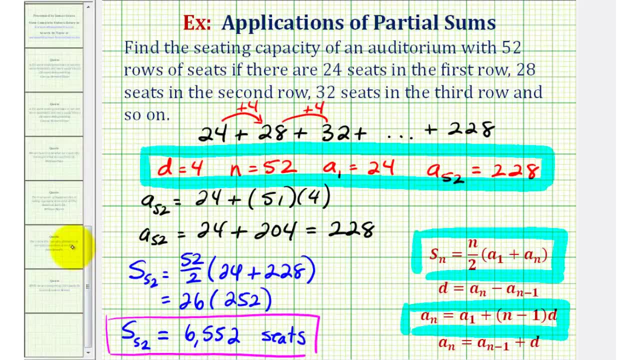 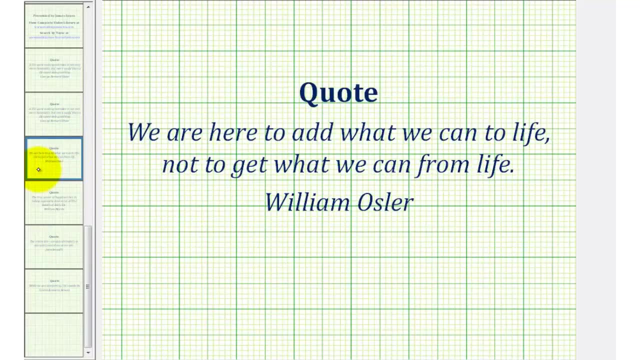 And this would be the number of seats. Okay, I hope you found this explanation helpful. Thank you for watching and I'll see you in the next video.